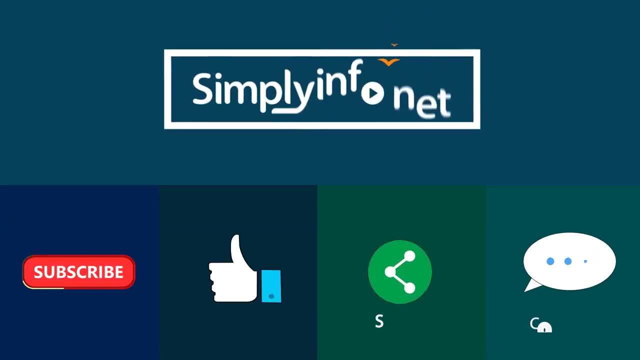 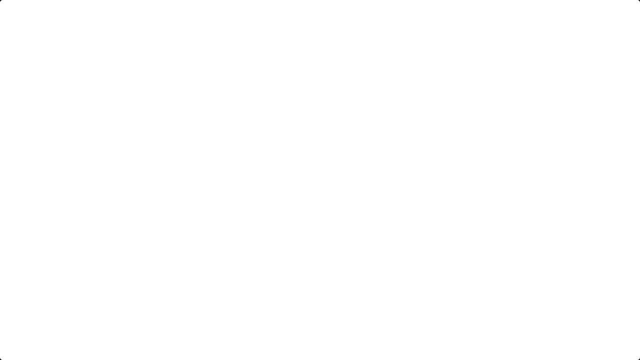 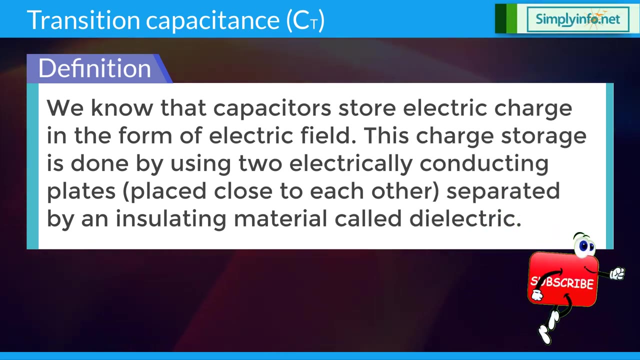 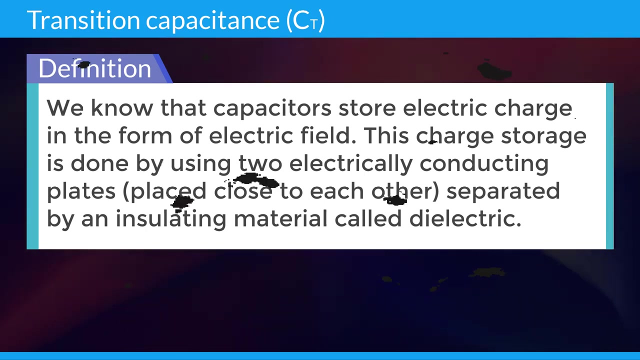 What is Transition Capacitance? Transitions Capacitance: We know that capacitors store electric charge in the form of electric field. This charge storage is done by using two electronically conducted plates placed close to each other, separated by an insulating material called dielectric. The conducting plates or electrodes of the capacitors are: 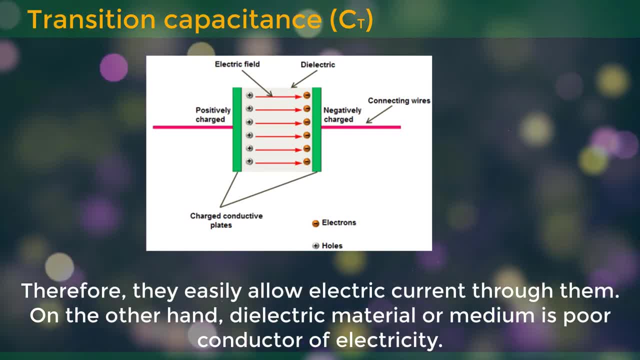 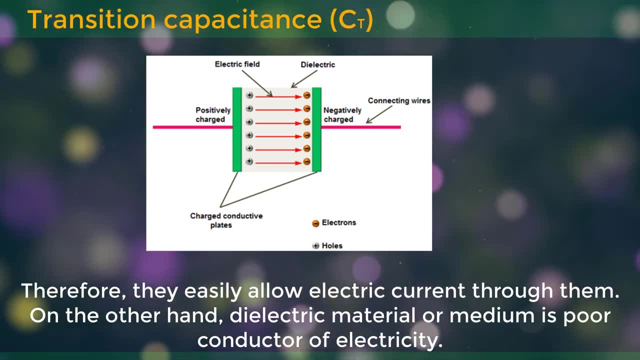 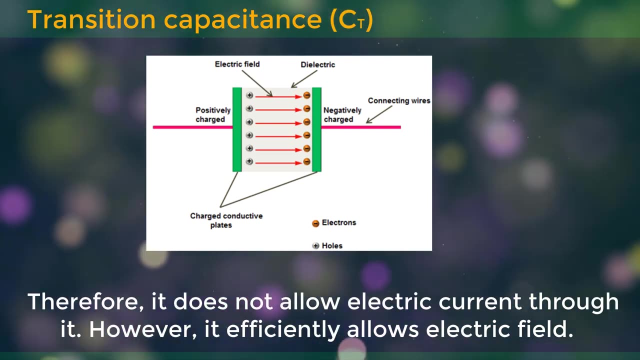 good conductors of electricity. Therefore they easily allow electric current to pass through them. On the other hand, dielectric material or medium is poor conductor of electricity. Therefore it does not allow electric current through it. However, it efficiently allows electric field. When voltage is applied to the capacitor, charged carriers start flowing. 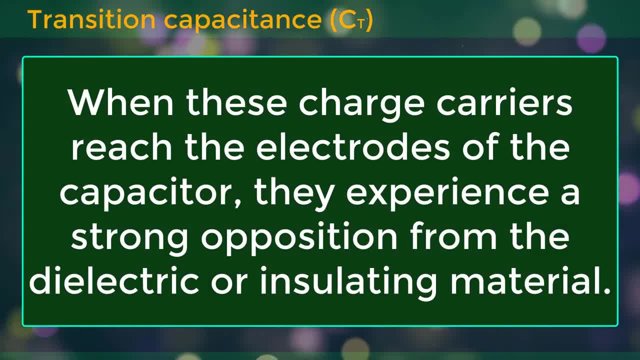 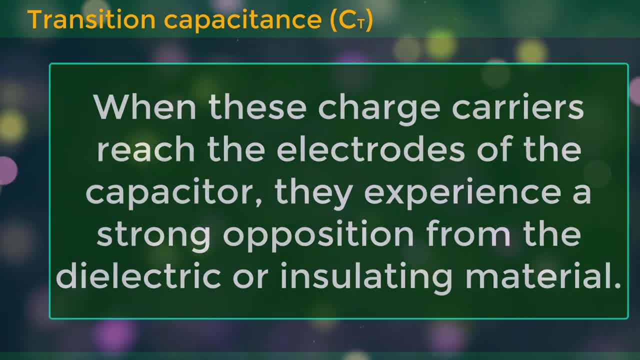 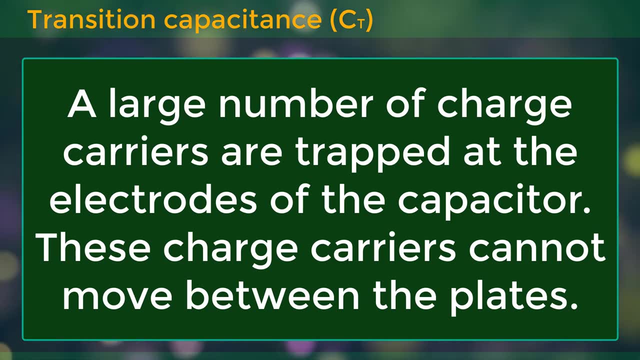 through the capacitor. When these charge carriers reach the electrodes of the capacitor, they experience a strong opposition from the dielectric or insulating material. As a result, a large number of charge carriers are trapped at the electrodes of the capacitor. These charge carriers cannot. 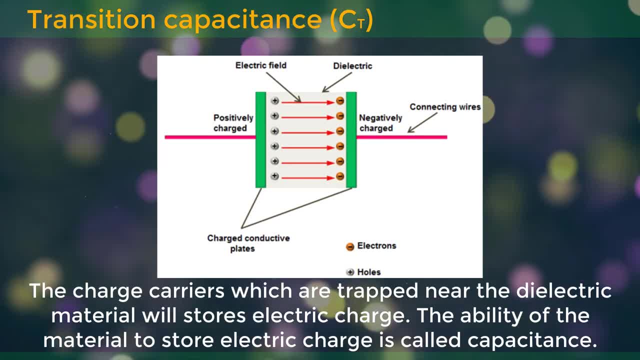 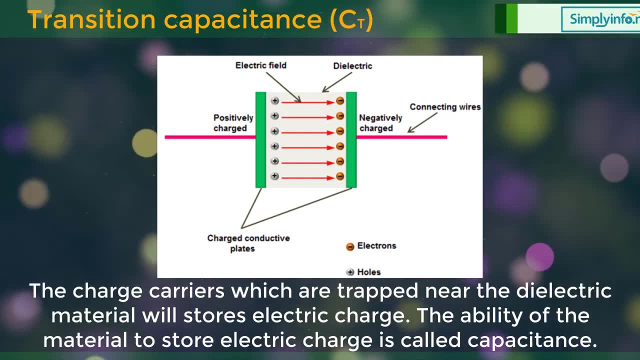 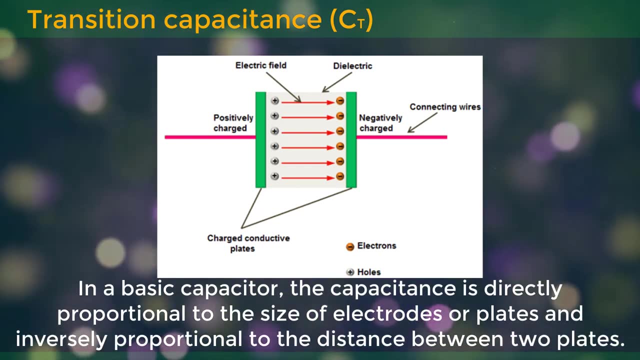 move between the plates. The charge carriers which are trapped near the dielectric material will store electric charge. The ability of the material to store electric charge is called capacitance. In a basic capacitor, the capacitance is directly proportional to the size of electrodes or 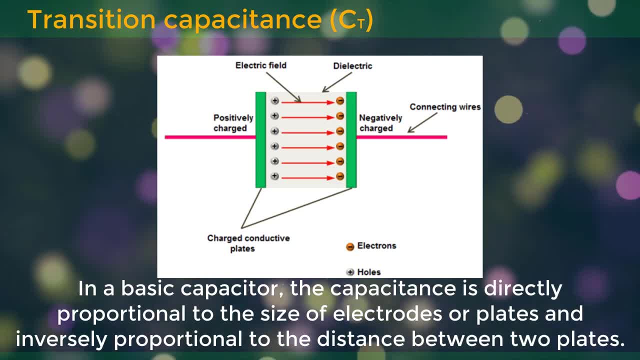 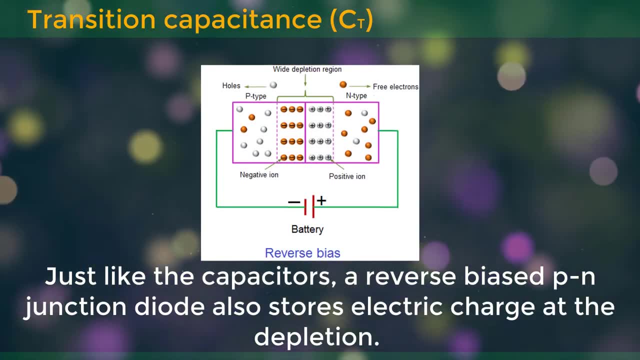 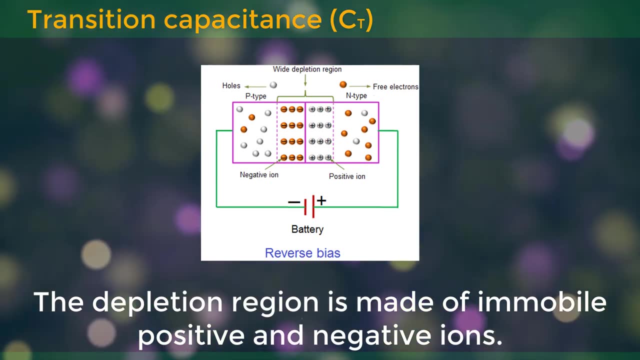 plates and inversely proportional to the distance between two plates. Just like the capacitors, a reverse biased P-N junction diode also stores electric charge at the depletion. The depletion region is made of immobile positive and negative ions. In a reverse biased P-N. 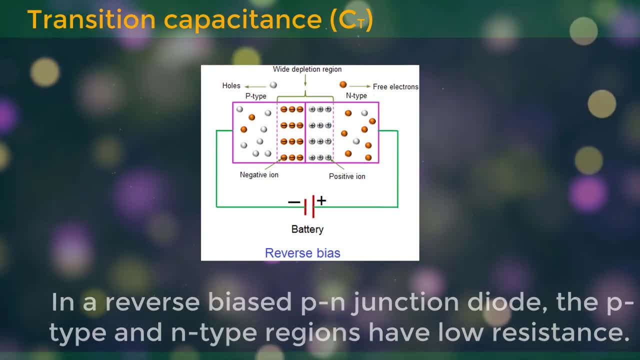 junction diode. the p-type and n-type diode are evenly divided so that they do not get into each other. This is because the state at which capacitors manifest on the electrode type regions have low resistance. Hence p-type and n-type regions act like the electrodes. 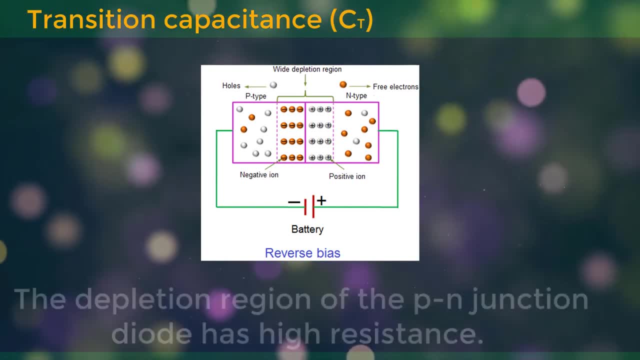 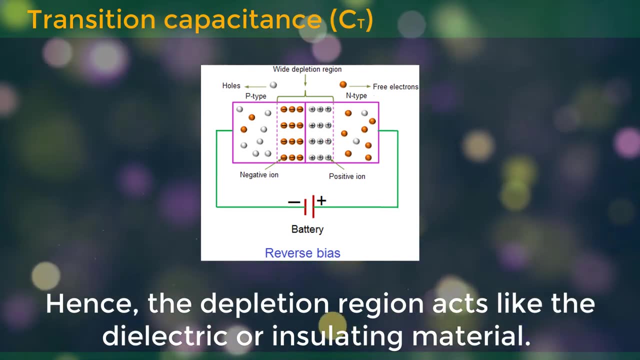 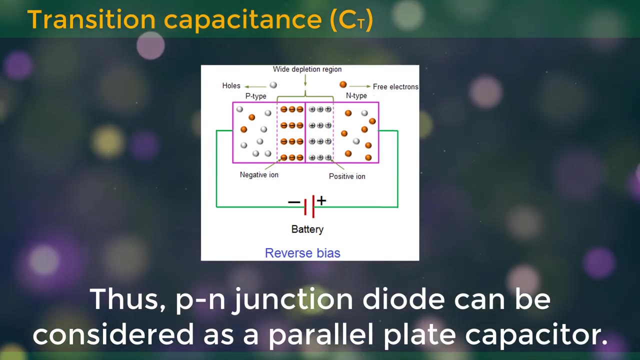 or conducting plates of the capacitor. The depletion region of the p-n junction diode has high resistance. Hence the depletion region acts like the dielectric or insulating material. Thus p-n junction diode can be considered as a parallel plate capacitor. 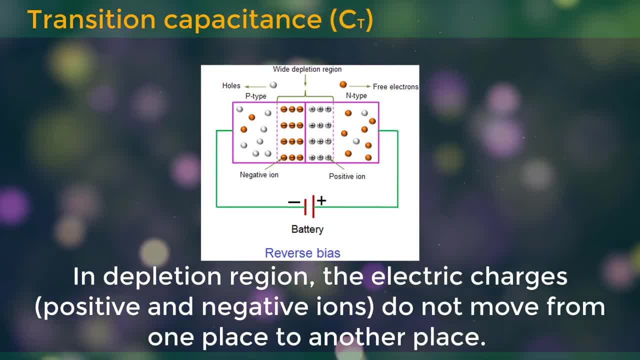 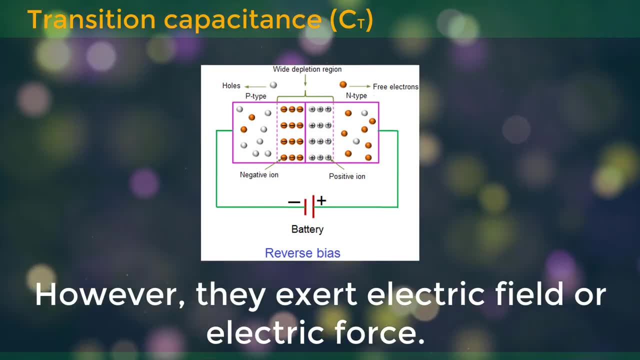 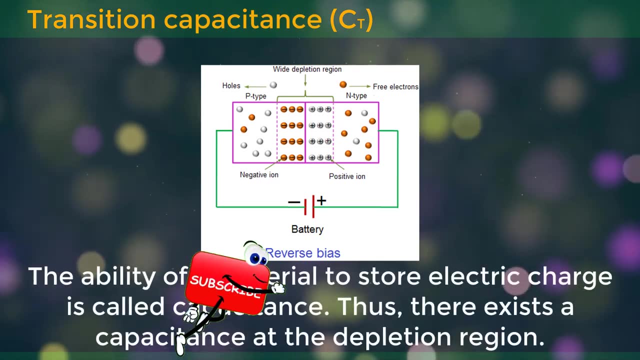 In depletion region. the electric charges, positive and negative ions- do not move from one place to another place, However, they exert electric field or electric force. Therefore, charge is stored at the depletion region in the form of electric field. The ability of 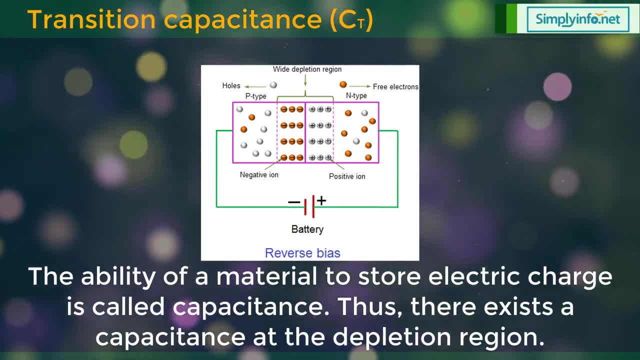 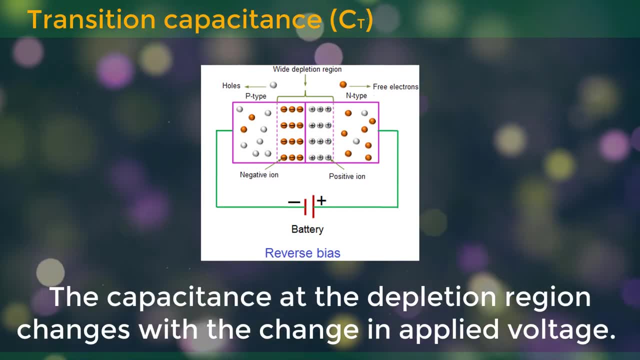 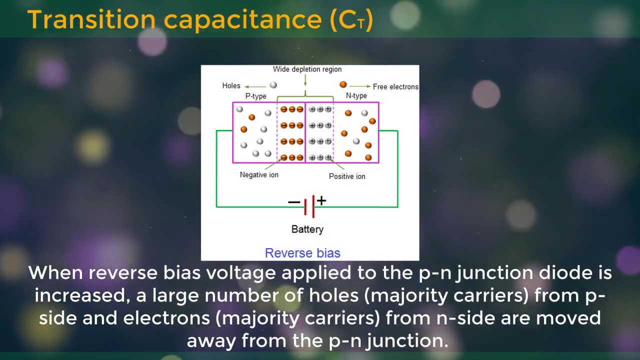 a material to store electric charge is called capacitance. Thus there exists a capacitance at the depletion region. The capacitance at the depletion region changes with the change in a p-n junction diode. When reverse bias voltage applied to the p-n junction diode is increased a large number. 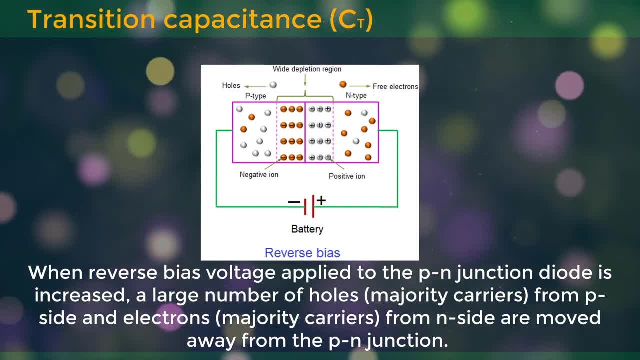 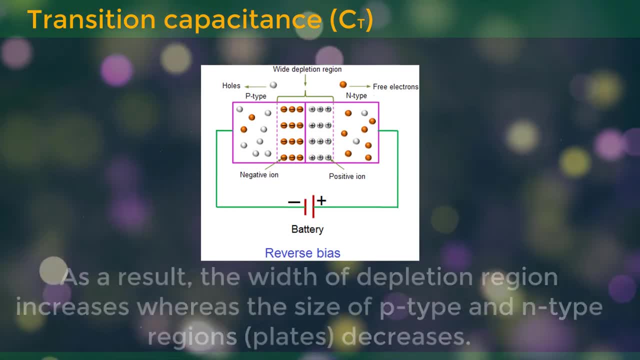 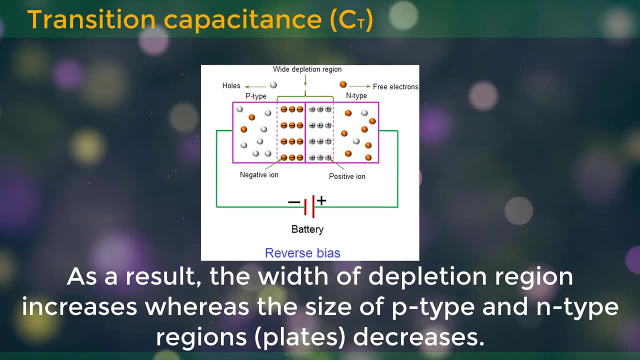 of holes. the majority carriers from the p-side and electrons minority carriers from n-side are moved away from the p-n junction. As a result, the width of depletion region increases, whereas the size of p-type and n-type region plates decreases. 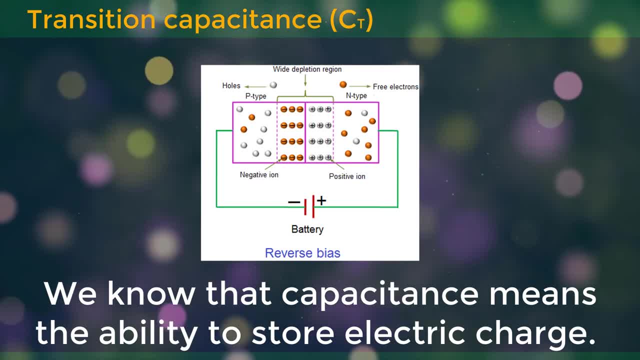 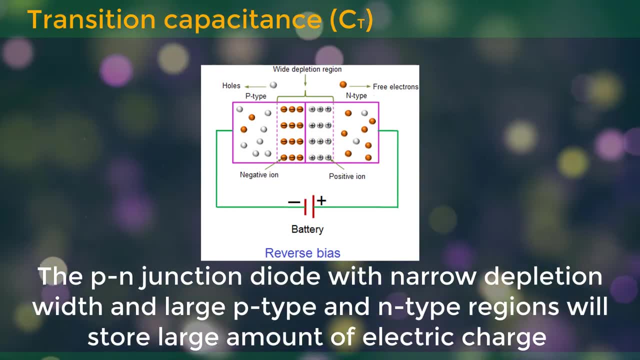 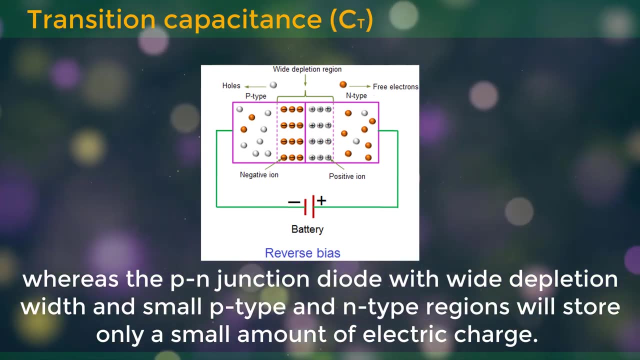 We know that capacitance means the ability to store electric charge. The p-n junction diode with narrow depletion width and large p-type and n-type regions will store large amount of electric charge, Whereas the p-n junction diode with wide depletion width and small p-type and n-type regions will store only a small amount of electric. 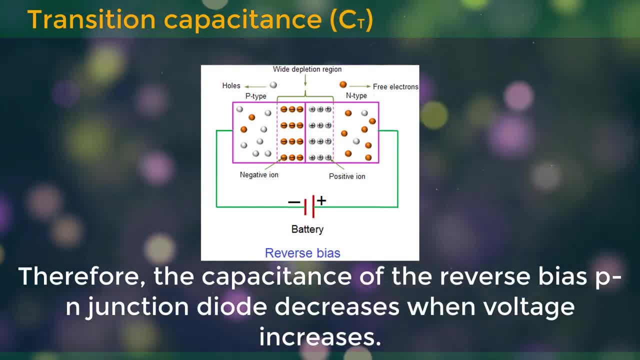 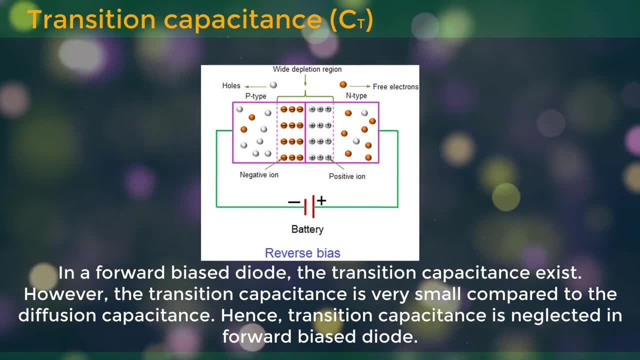 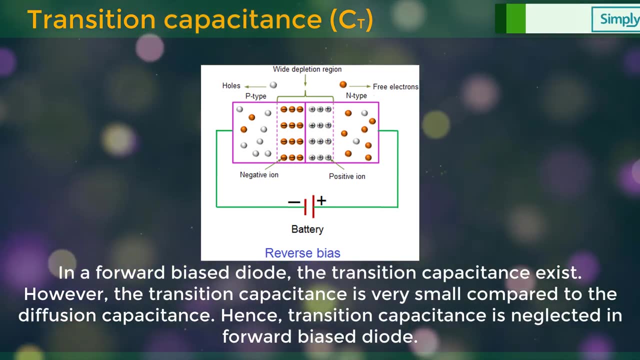 charge. Therefore the capacitance of the reverse bias p-n junction diode decreases when voltage increases. In a forward biased diode, the transition capacitance exists. However the transition capacitance is very small compared to the diffusion capacitance. Hence transition capacitance is neglected in forward biased diode. 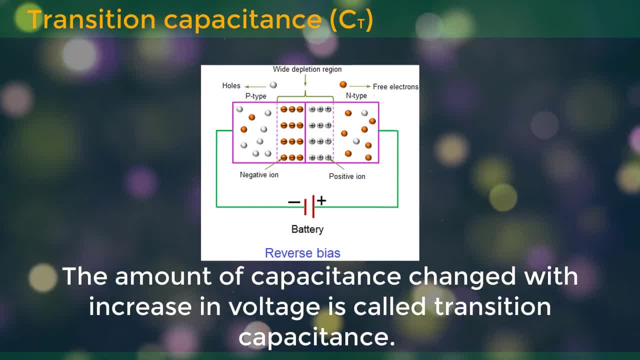 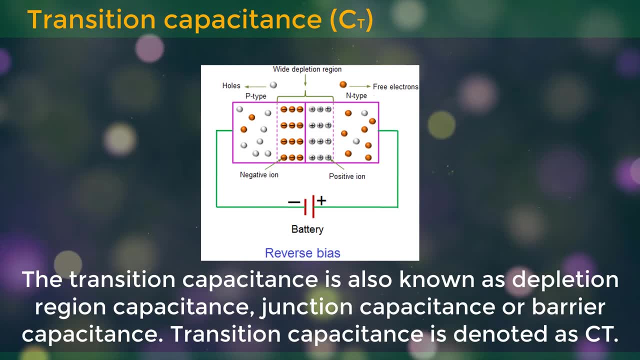 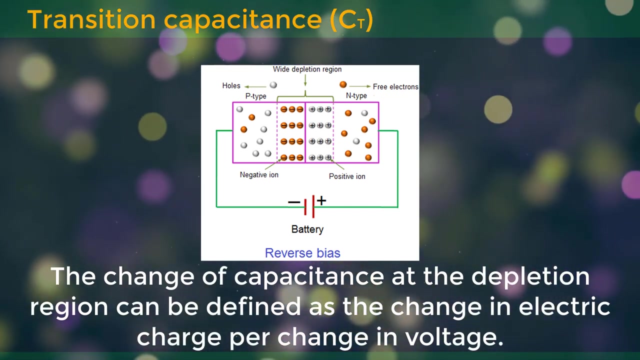 The amount of capacitance changed with increase in voltage is called transition capacitance. The transition capacitance is also known as depletion region capacitance, junction capacitance or barrier capacitance. The transition capacitance is denoted as Ct. The change of capacitance at the depletion region can be defined as a change in electrical 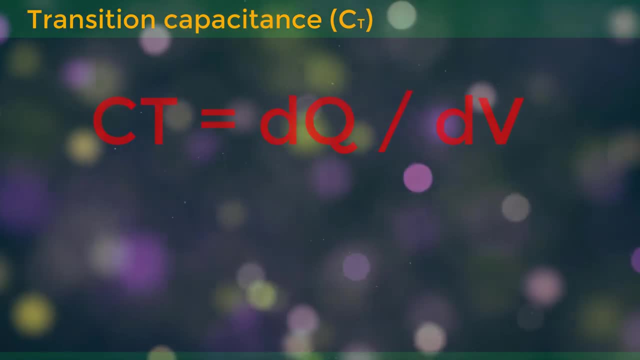 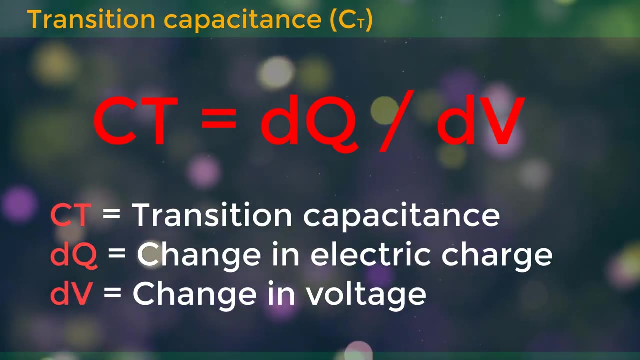 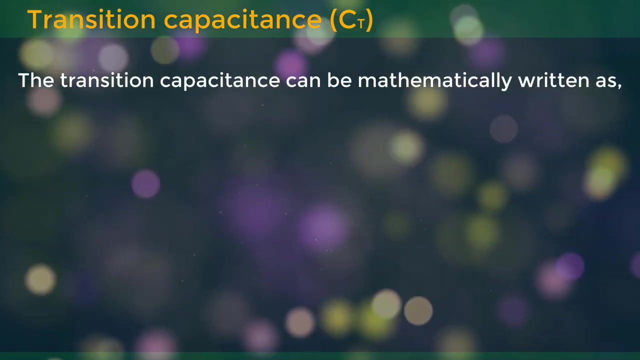 charge per change in voltage. So Ct equals to dq by dv, where Ct stands for transition capacitance, dq- change in electric charge, dv- change in voltage. The transition capacitance can be mathematically written as: Ct equals to a plus on a to the.